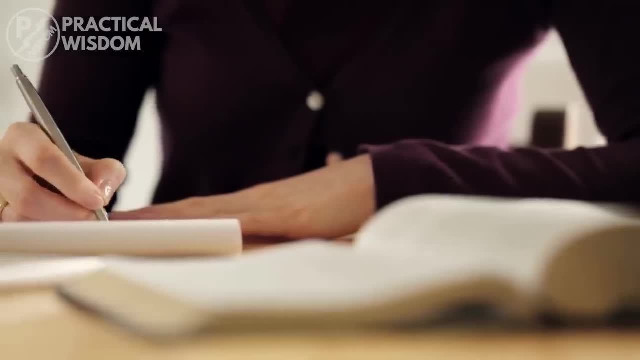 probably not doing it. Basically, it should always be a priority. Basically, it should always be a priority. Make sure that every single penny you spend is clearly accounted for. The basic goal of expense tracking is to find and get rid of inefficient spending patterns in your financial 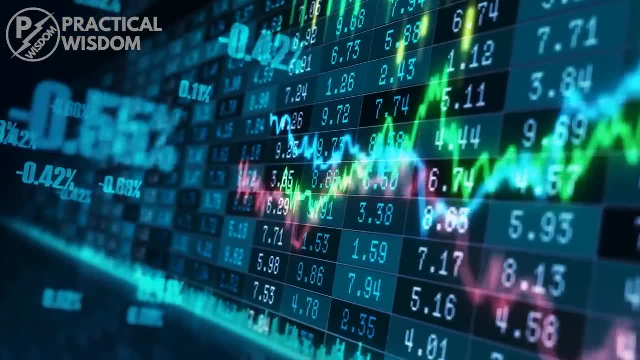 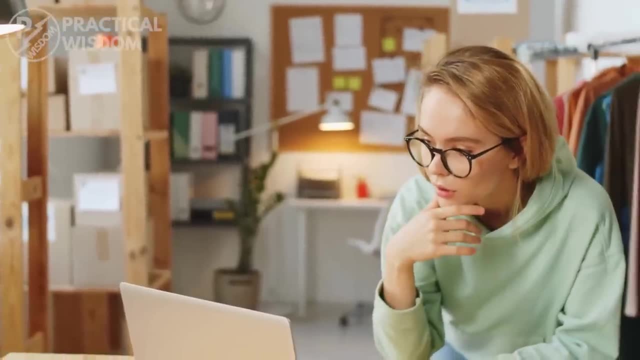 life. Additionally, maintaining control over your finances and encouraging better financial practices like saving and investing will come from continuously keeping track of your costs. Basically, in the words of Peter Drucker, if you can't measure it, you can't manage it. 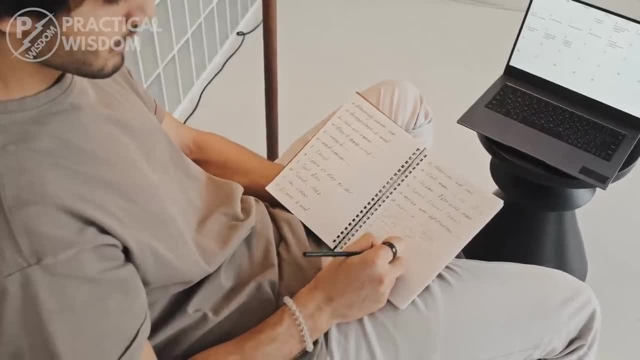 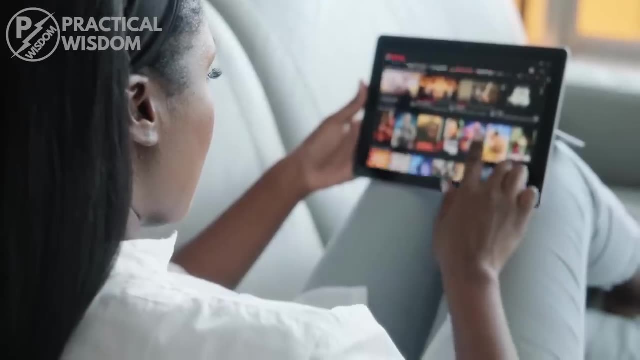 So this is what you should do to get in control of your spending habits. first and foremost, You should analyze your categories of spending to determine which are the most crucial. Perhaps you might even find out that you've been paying for a subscription that you're not using. 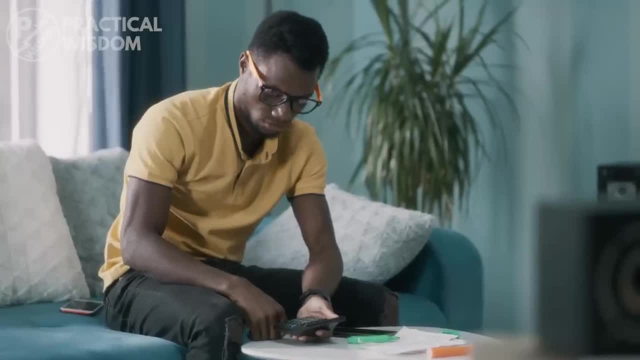 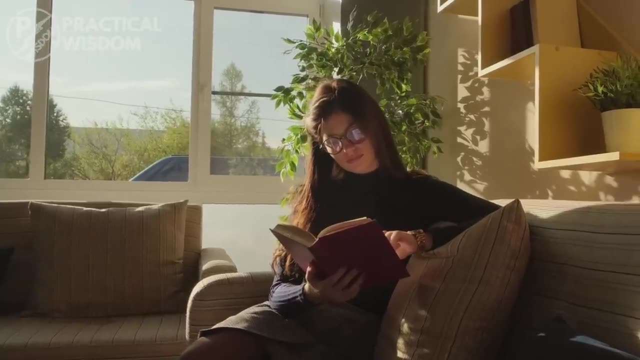 I know I have, and maybe you are too. Most people consider that cutting back on these non-essential expenses is a wise approach to saving money. You might also want to go for activities that are less expensive, now that you can see where your money is going, And on top of, 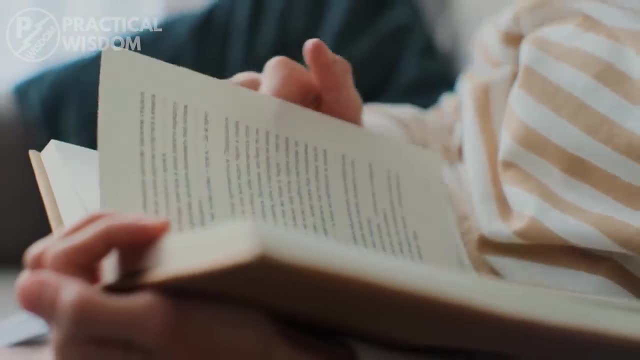 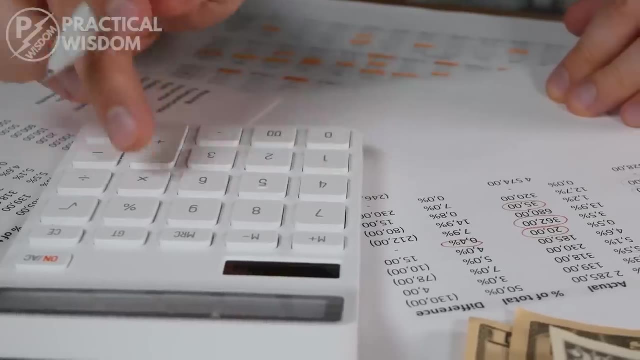 saving money. you'll be getting educated on some of the topics you'll be reading about, So there really isn't much to lose by doing this. 2. Make a budget. I never understood why most people didn't have a budget until recently. 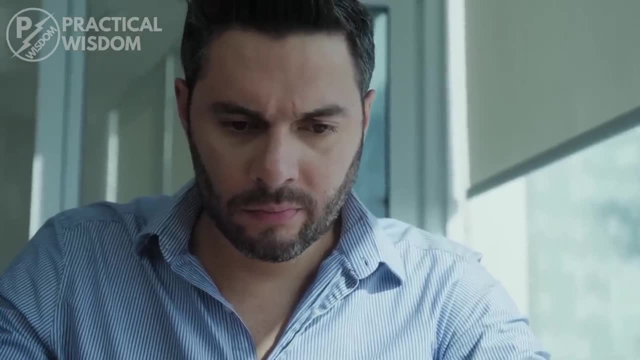 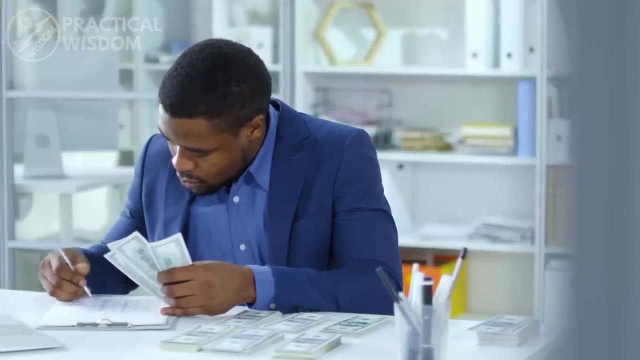 You see, most people are worried about all the paperwork to be done to complete a budget. Well, in truth, it's a lot of work, but it is most certainly worth it. You see, you should look at budgeting from a different angle. Look at the positives and look. 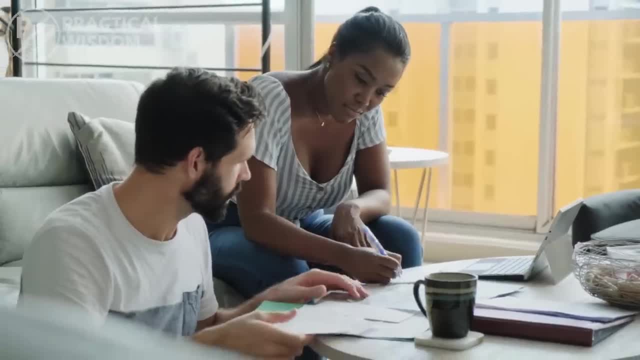 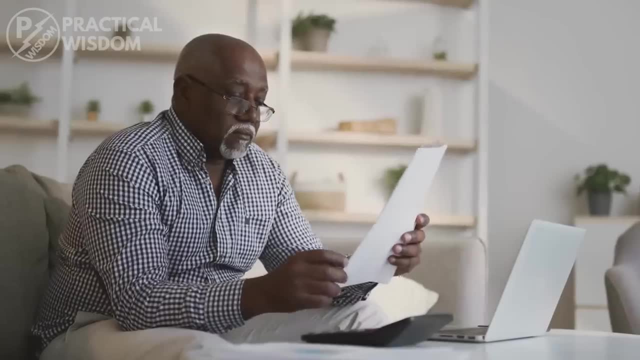 at how much is it going to benefit you, And once you've got a rhythm going, make sure you stick to it. I've found this to be the only way that works, so make sure you don't lose the momentum If you create a budget and then store it away in a file or folder on your bookshelf or filing cabinet. 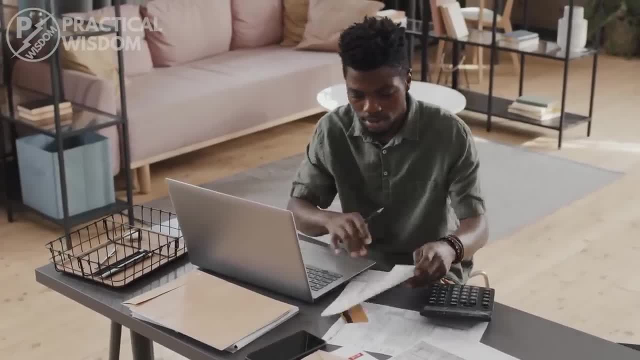 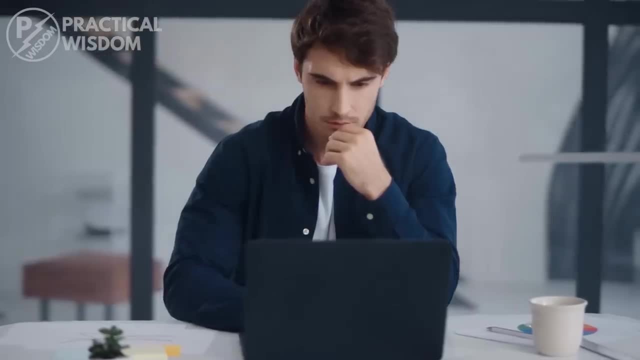 it's simply worthless, So make your constantly updating and reviewing it. You can also use digital apps and software to make this task a lot easier. There are a bunch of really good free ones online which you can find with a quick search. 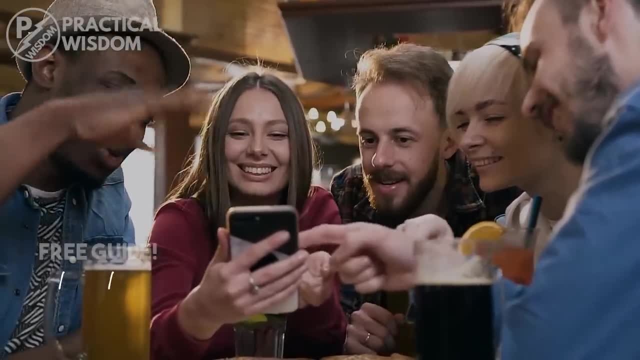 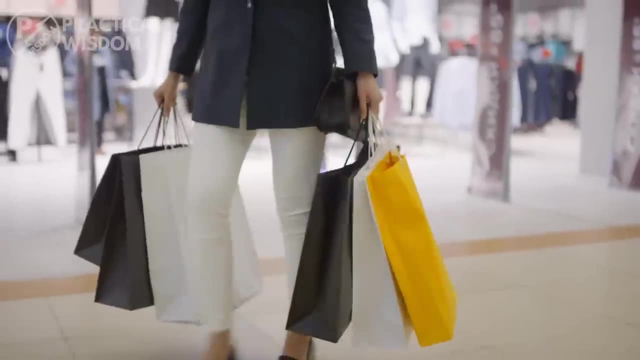 And, if you're interested, I created a free savings and budgeting guide which you can get with the link in the description. 3. Give yourself a limit on unbudgeted spending: Buying something in the spur of the moment that you hadn't. 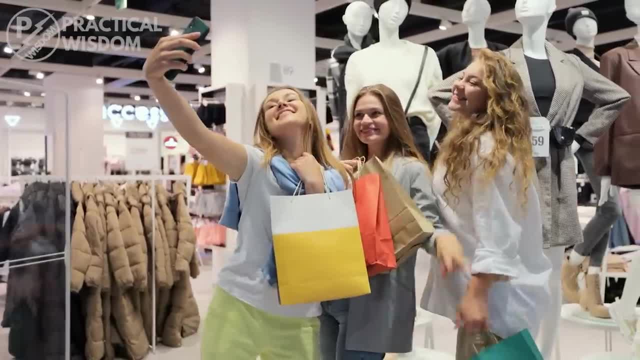 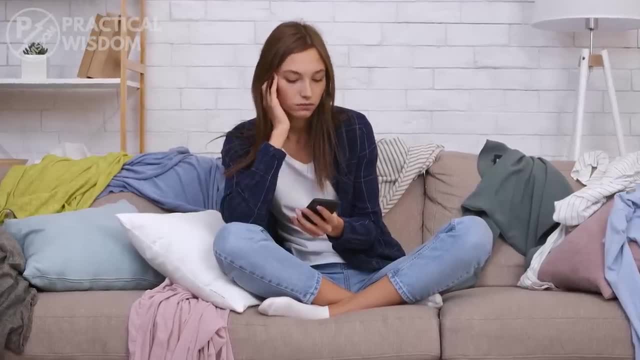 budgeted for can be enjoyable and emotionally satisfying. Literally everyone knows that. However, that emotional high may pass quickly, leaving you with impulse purchases you don't actually need or want. If this is you, then the bitter pill to swallow is that this has to stop. 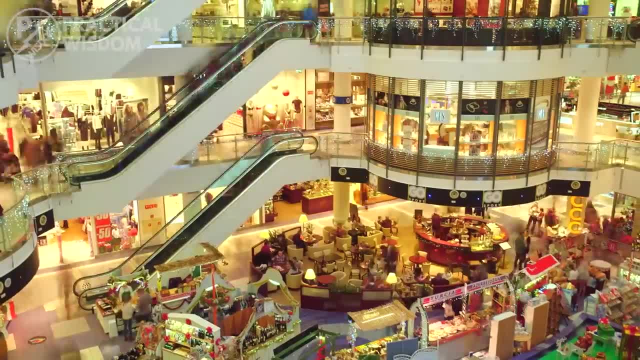 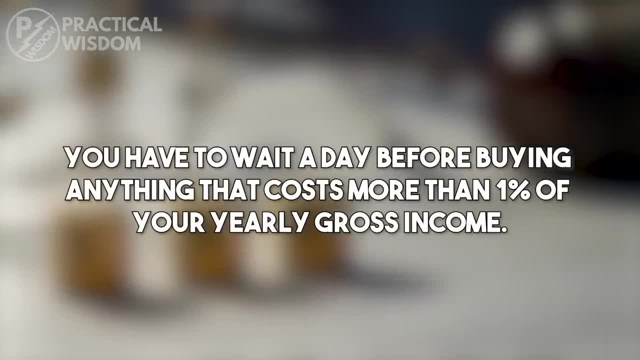 In fact, it's the entire opposite of good money habits. Next time you're in the mall, try using the 1% rule for spending money. This rule states that you have to wait a day before buying anything that costs more than 1% of your yearly gross income. So if you make, $600 a year. the rule states that you need a day before making a purchase of over $600.. This guideline applies to discretionary spending on items you desire but don't require. Basically, the inner battle in your mind of do I really need this versus do I want this. 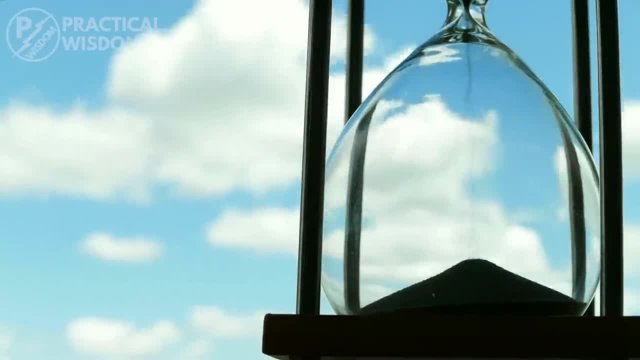 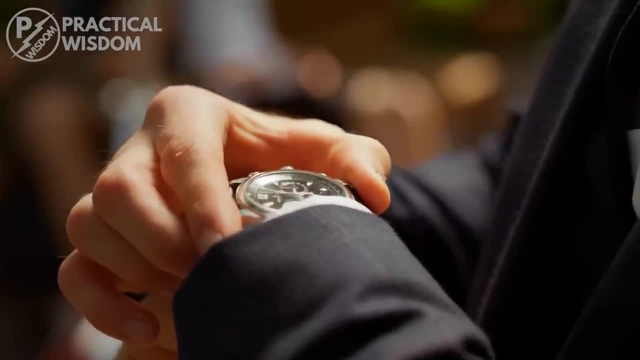 The 24-hour cooling off period gives you time to reconsider your purchase. Why not take an additional day to consider if you actually need it? After 24 hours you might not anymore. So next time you go shopping, remember what that guy from. 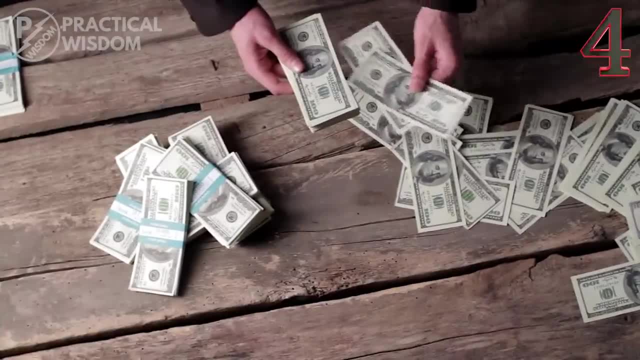 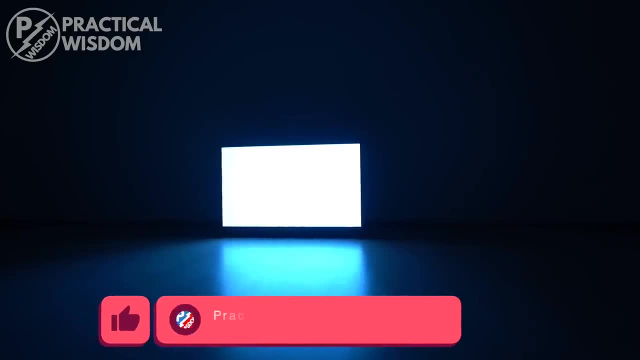 Practical Wisdom told you to try. 4. Save for big purchases. Seeing a beautiful $4,000 advertisement of a stunning 90-inch flat-screen 8K television, I mean imagine the things you can see on that TV- does not mean that you should immediately. 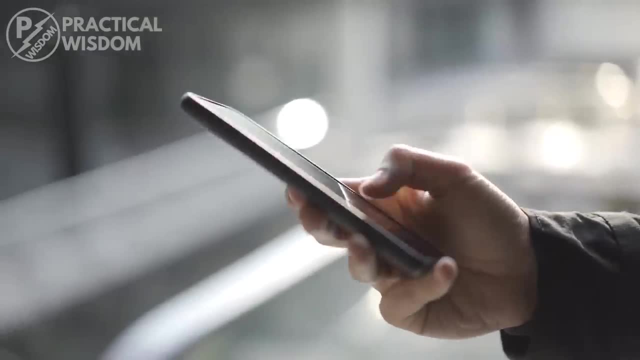 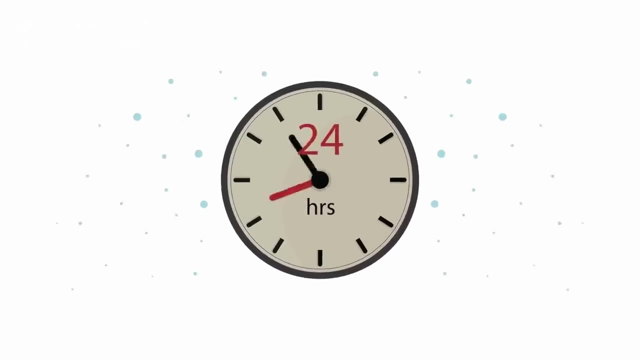 pick up your phone and credit card and start dialing the number on the screen. That's a really bad idea. Remember the rule that the guy from Practical Wisdom told you about The 24-hour one. Remember that. So experts suggest that if you really want that big TV, 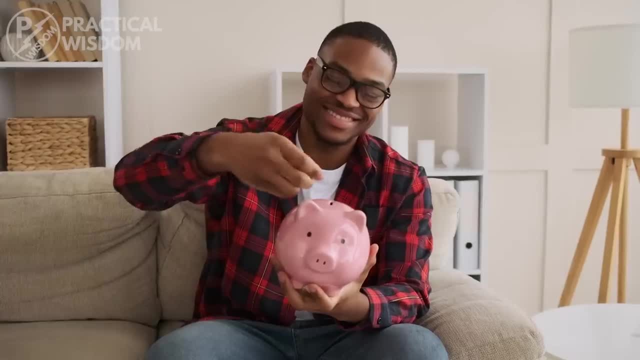 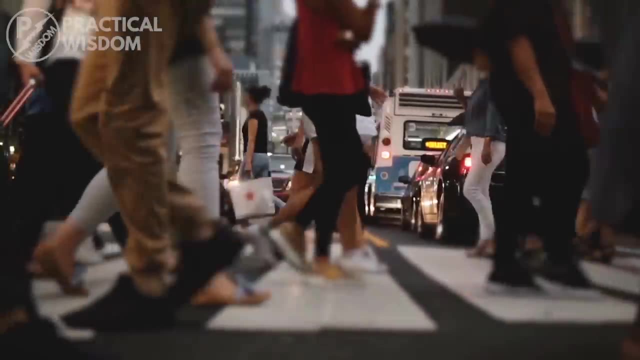 then it's best that the money comes from your savings account, Which is dedicated for such purchases, Not a credit card loan, unless you have a really good plan to pay back the money, which 99% of people don't. Also, there are countless 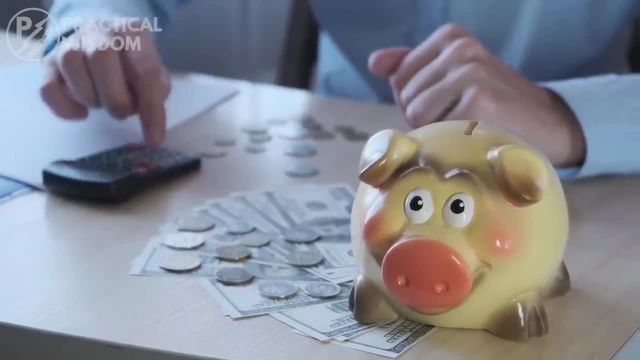 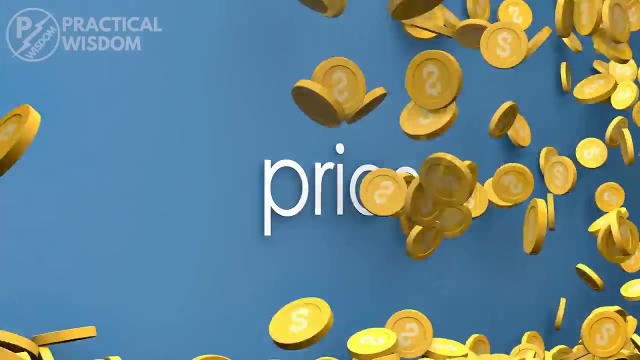 advantages that come with saving for a big or expensive purchase. You may be able to negotiate a cheaper price or, at the very least, better financing conditions. If you save up and pay cash, the price could drop as well. Additionally for a larger purchase. 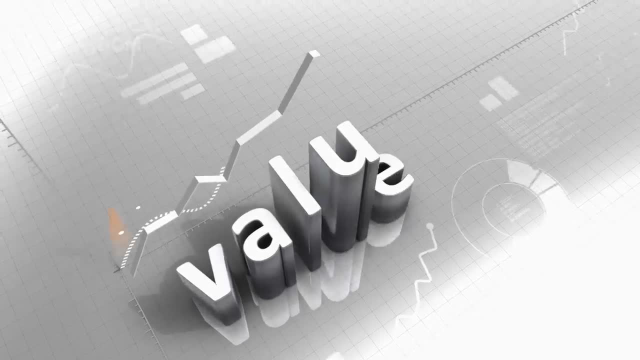 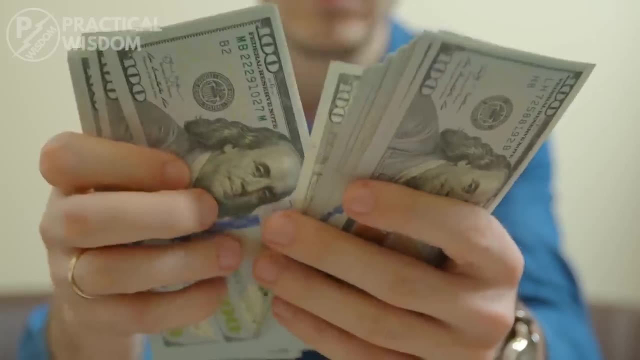 getting a loan may make more sense, especially if it's an item with appreciating value, like a home, or if it prevents you from taking money out of your savings or investment account, As paying in cash for the big, expensive TV might leave you with little to spend. 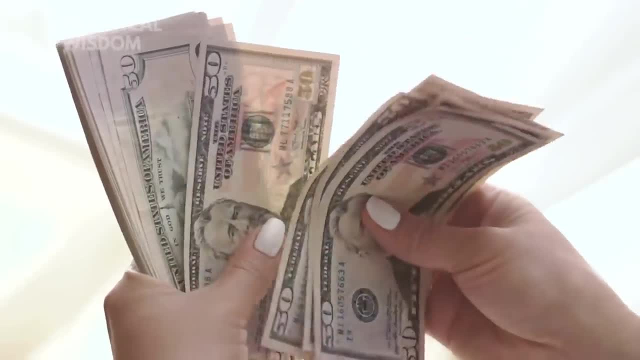 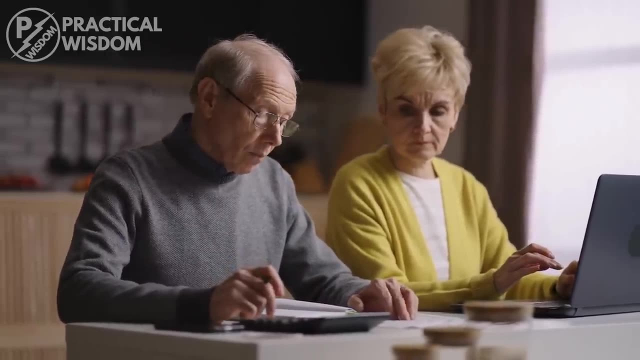 therefore, it's wise to save up for a while before you buy the products you need or desire. Therefore, it's sensible to start saving for that specific thing so that your daily life is not disrupted. 5. Read books about finance. It's true when they say that if you want to hide something, just put it on paper. 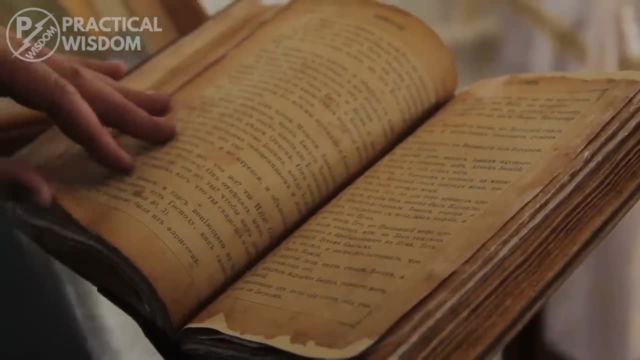 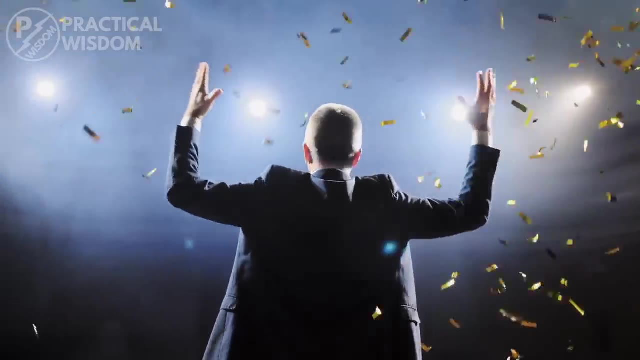 The sad truth is that most people never bother to read. You see, some of the things that you read people choose to ignore, such as the information contained in books, has a good chance of making them successful if they bother to read them. 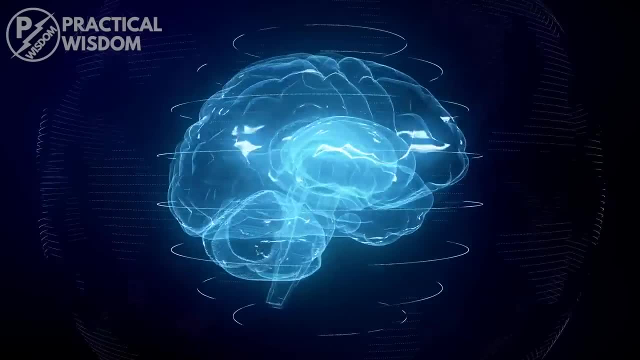 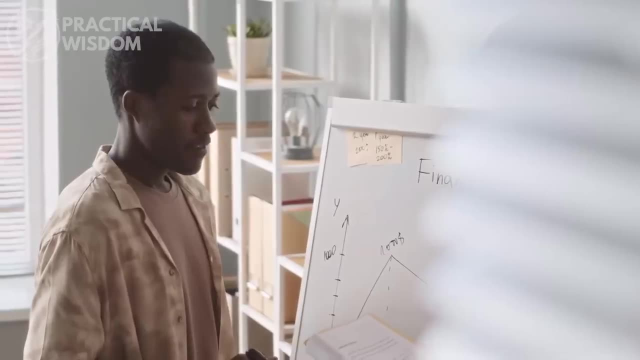 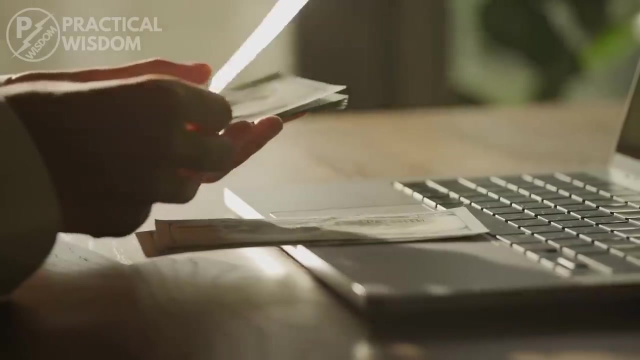 Learning is a continuous process and the more you do it, the sharper your skills become. The ability to make wise financial decisions is the chief advantage of financial literacy. It gives us the information and abilities we need to properly manage our finances, including budgeting, saving, borrowing and investing. As a result, 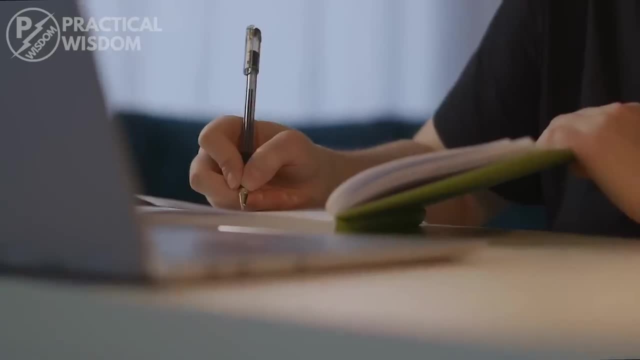 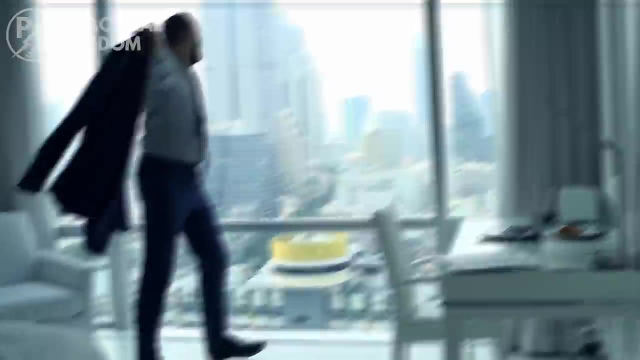 we're better positioned to meet our financial objectives and establish financial stability. It's kind of like a superpower and it really puts you in a comfortable situation knowing that you're in control of your financial destiny. 6. Lower your monthly bill. 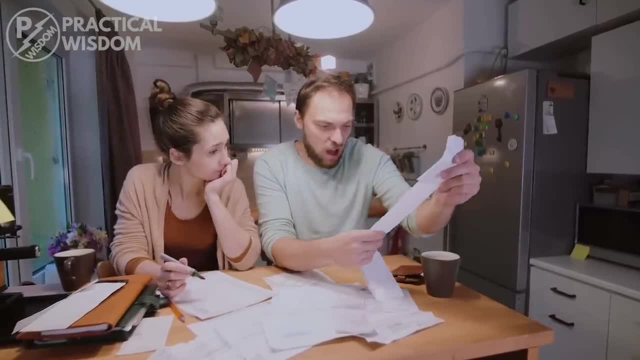 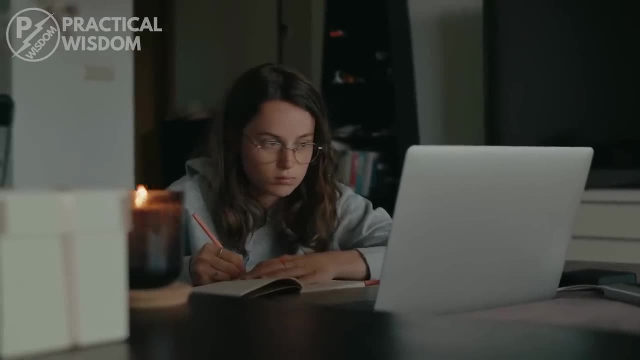 Cutting your monthly spending is one of the simplest ways to gain control of your money. While you might not be able to cut back on certain permanent costs, like rent or vehicle payments, without making significant lifestyle changes, you can cut back on variable costs like clothes or entertainment. 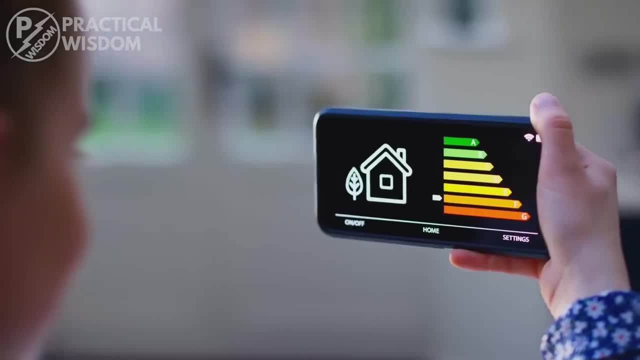 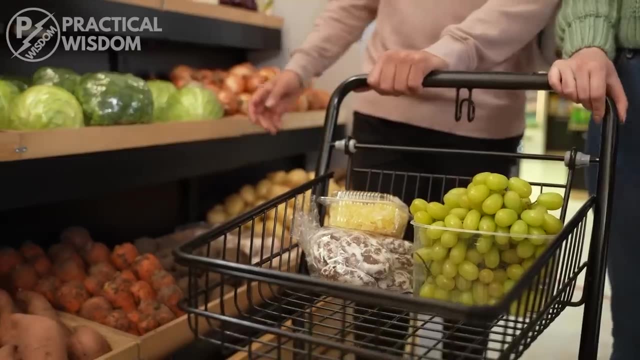 by being adaptable and thinking sparingly To begin saving on things like your energy bills. you may, for instance, use less power, pick a different life or home insurance company, or shop for your groceries at bulk discounts. Additionally, you shouldn't accept a loan just 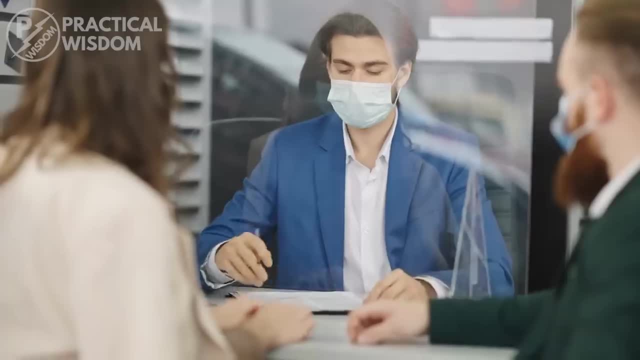 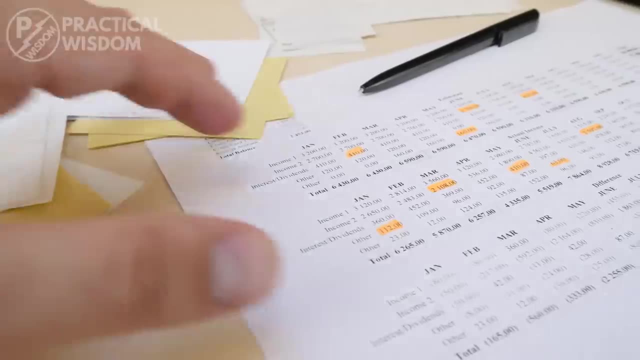 because your salary and credit make you eligible for one. Many people believe that the bank will not give them a credit card or a loan that they cannot afford, but the bank is only aware of the income you've disclosed and the debts shown on your credit report. The bank is unaware of any. 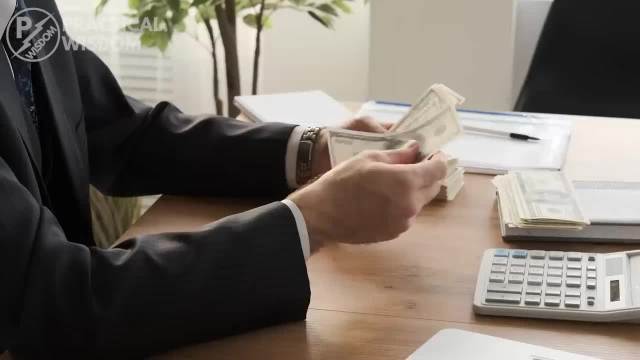 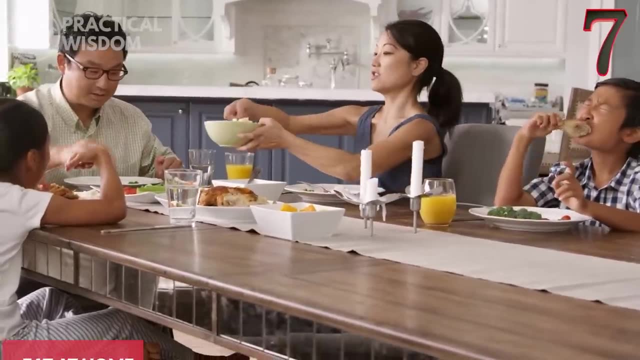 other commitments that would make it difficult for you to make timely payments. Based on your income and other monthly responsibilities, you must therefore determine if a monthly payment works for you. 7. Eat at home. Meals prepared and consumed at home may be quite cost-effective. All you have to do is reduce your 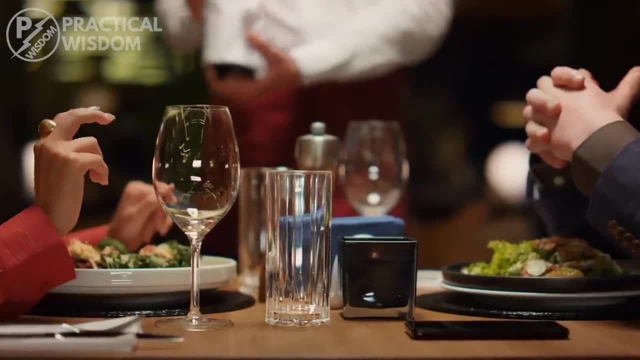 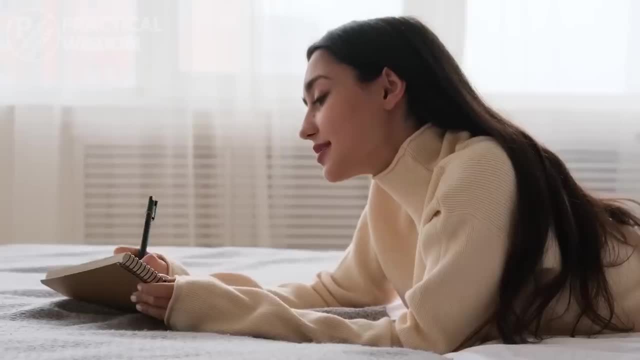 reliance on take-out. The odd indulgence at a fancy restaurant is okay, but starting to cook at home or carrying packed lunches to work, rather than dining out every day, might save you money. Making a weekly food plan may make it simple: Plan your meals for the coming week and then. 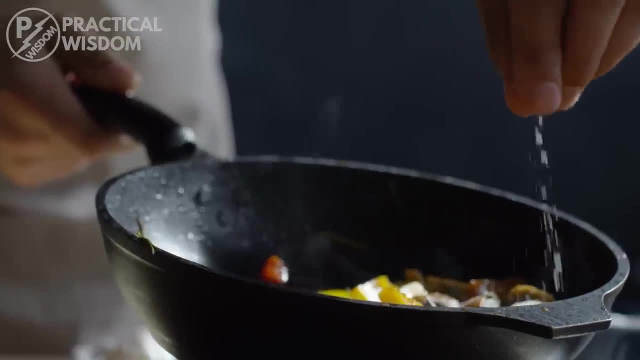 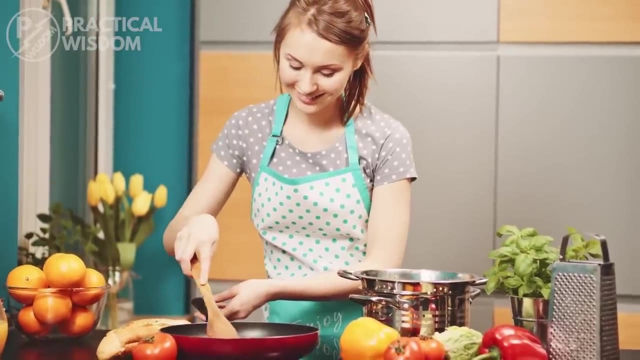 stick to them. Even for those who don't consider themselves to be cooks, the internet provides a seemingly limitless array of culinary and recipe-advantaged food options for you to choose from. Begin by making at least one meal a week at home. Bring your lunches to work, starting next. 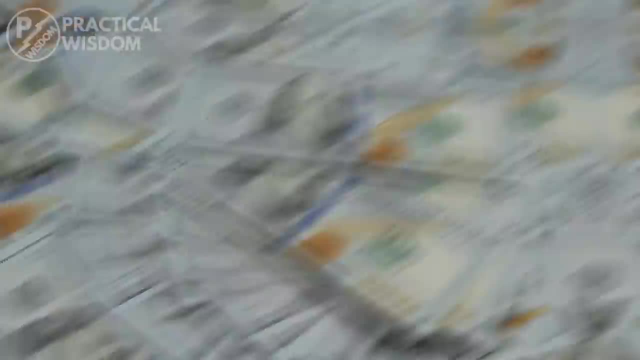 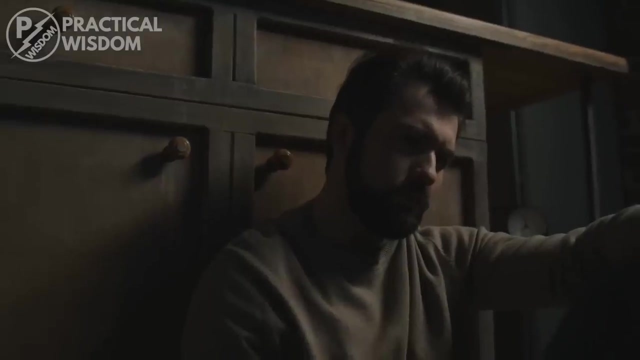 week, You might be amazed by how much money you can actually save. 8. Pay off your debt. Carrying a lot of debt, especially on high-interest credit cards, is one of the costliest mistakes you can make If you want to improve your financial situation and open up new. 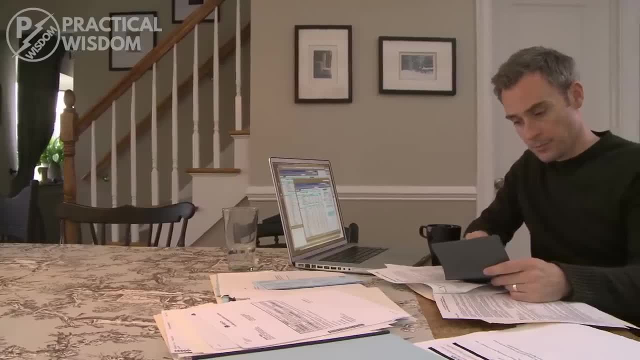 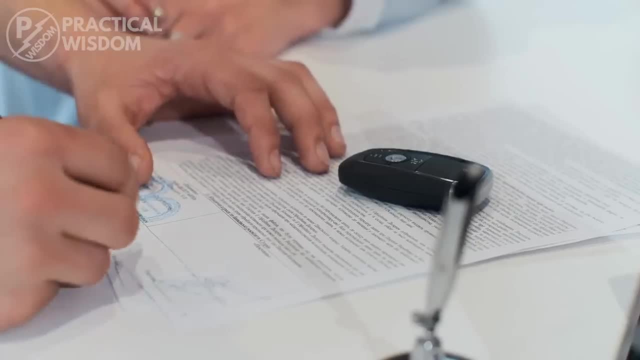 financial opportunities. pay off your debt as soon as possible. If you're the forgetful type, you should list off all your existing debts, including credit card debt, student loan debt and vehicle loans, and determine the minimum payments you must make to stay on top. 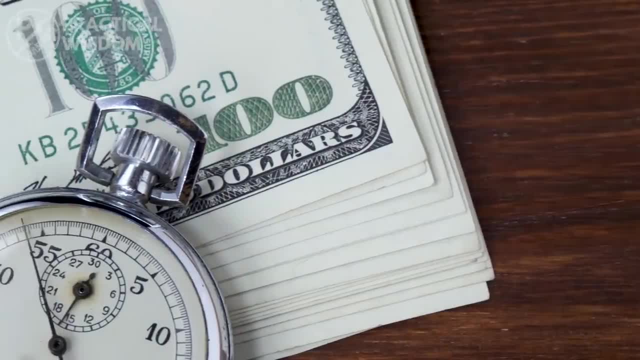 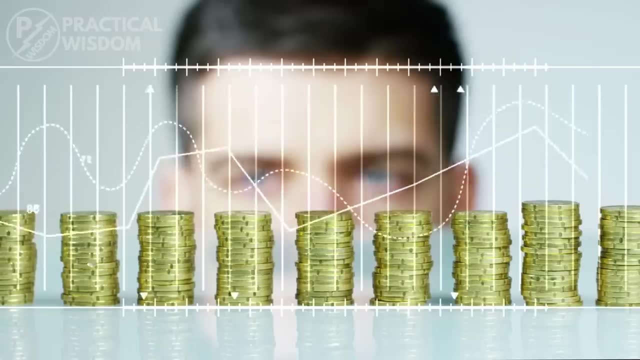 of each of them. Making minimum payments will not get you out of debt quickly, so consider your fixed costs and how much of your discretionary spending budget you can set aside for debt repayment. Additionally, you can try to lower the interest rate on the debt by requesting a lower. 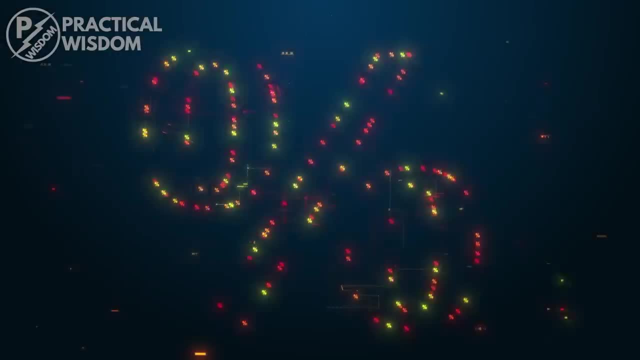 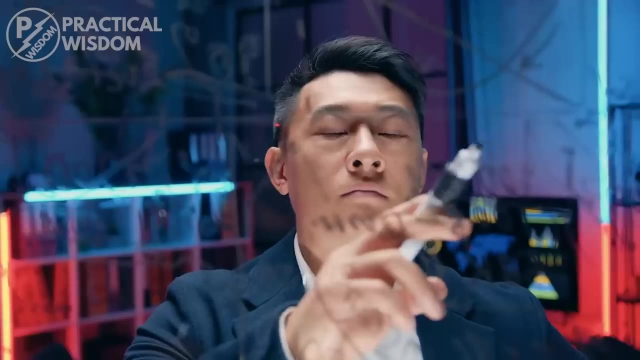 rate from the issuer, merging several loans into one or moving high-interest debt to a low-interest credit card, such as a balance transfer card, to lower the overall interest rate Afterward. create and develop responsible spending practices to pay off the debt as rapidly as possible. 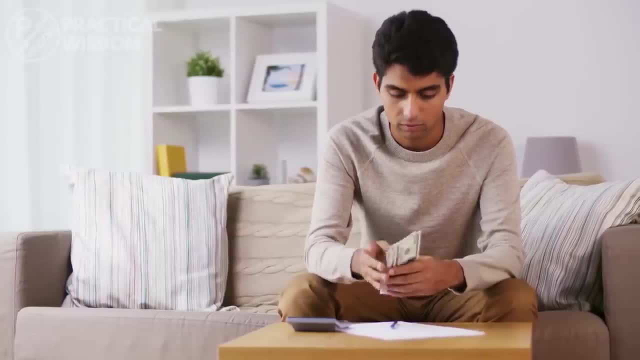 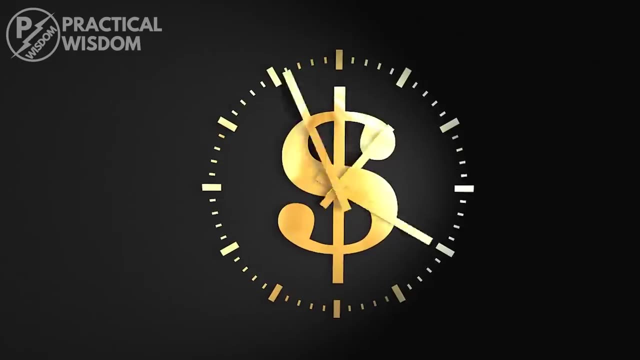 Your monthly budget will be larger the faster you pay off your debt. As I previously said, paying off credit card debt must be a top priority. Unlike your automobile or house payment, it increases with time and is hard to cut back on. 9. Stop using credit cards. 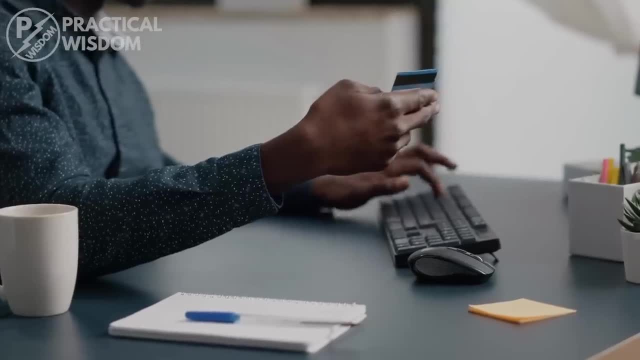 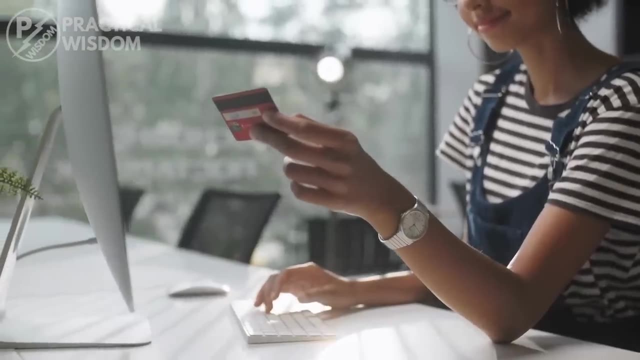 Credit cards are a great and handy tool to have. They're a lifesaver when needed and they do a great job getting that credit score up. However, for some people, their lack of self-control and an easy and available remedy to their problems in the form of a credit card means that they quick dig themselves into 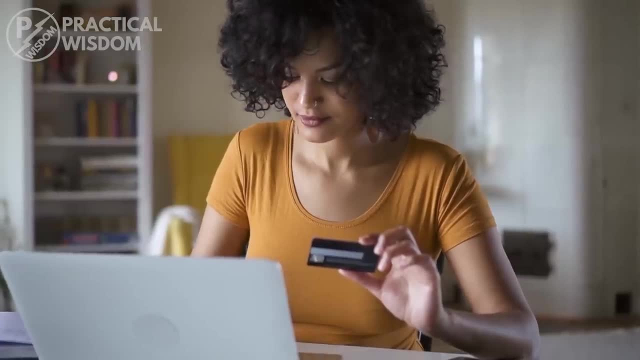 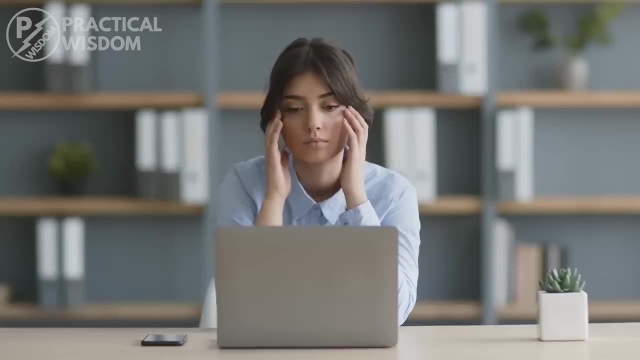 disaster. You could be depending too much on your credit cards. if you're having trouble making ends meet each month, If you continue using your credit cards as a crutch to get by, you'll soon find yourself in debt. Your ability to pay your expenses, save for retirement or pursue other. 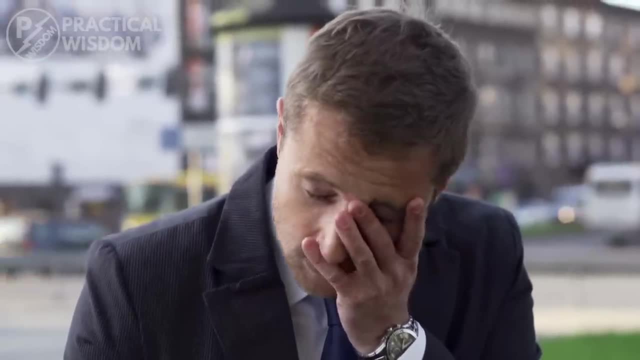 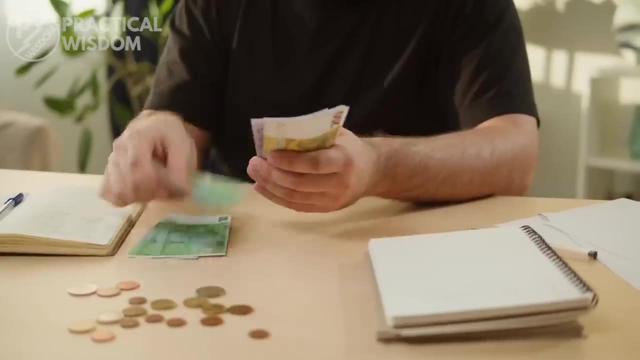 financial objectives will be constrained as a result of this. So stop using your credit cards. if you genuinely want to take charge of your money, to prevent accumulating more debt, in addition to creating a budget so that you don't have to use credit, Try switching to cash or debit cards. 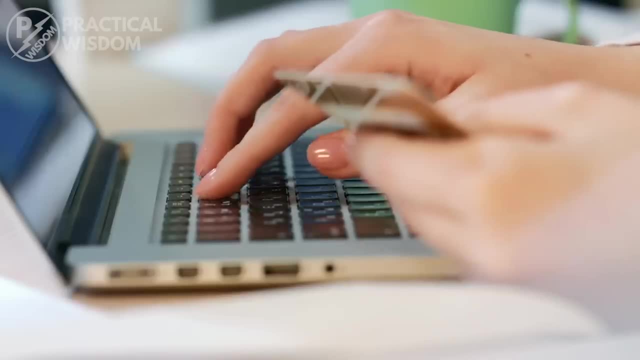 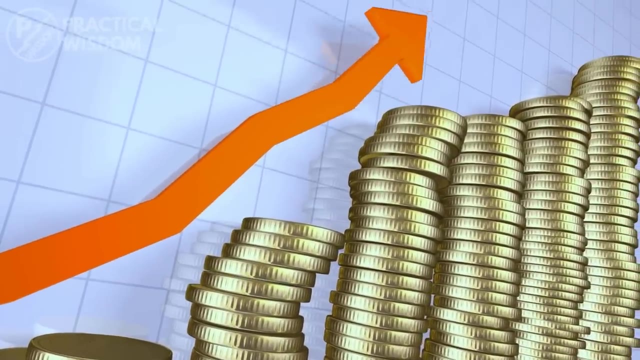 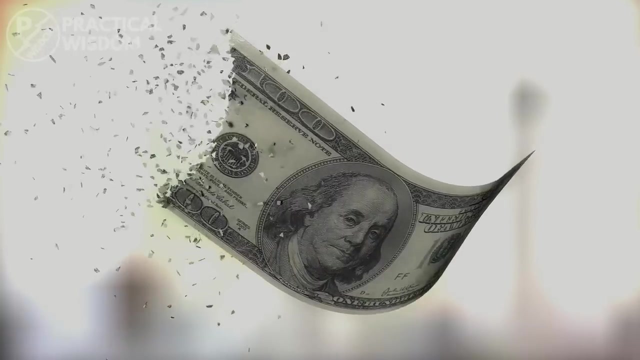 opening a short-term savings account and using funds from it for major purchases or leaving your credit card at home. Credit cards have high interest rates that may quickly accumulate debt if not used wisely and can cause significant stress in the event of an emergency Because they feel like their money disappears too quickly each month. 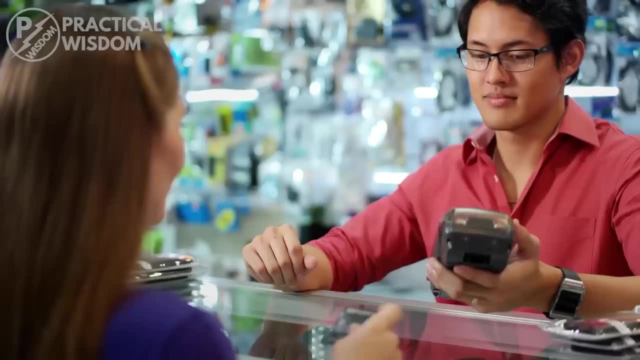 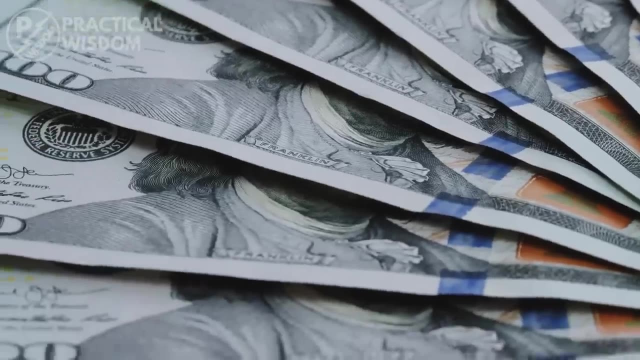 many people develop the bad habit of depending on their credit cards. They're tapped out and rely on their credit cards to get them through till payday after paying bills, food, rent or mortgage and other expenses. Instead of relying only on your credit cards to cover expenses, stop using them altogether until you develop the wisdom and 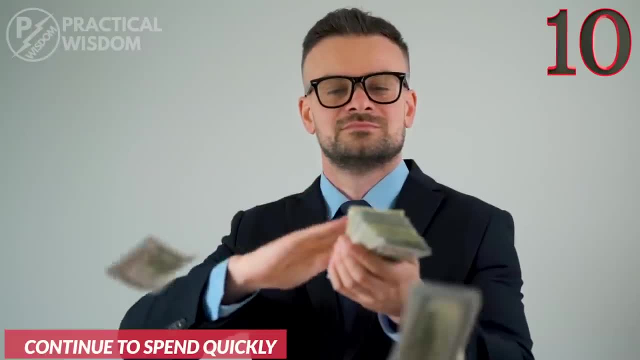 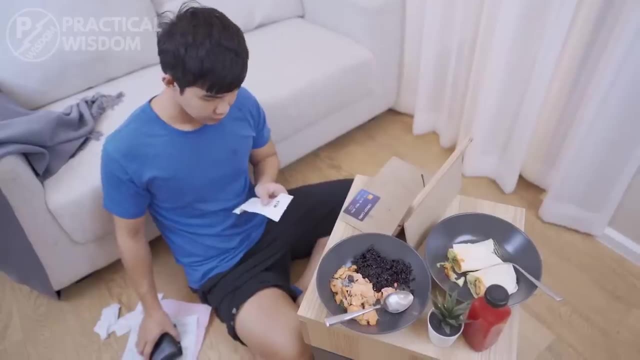 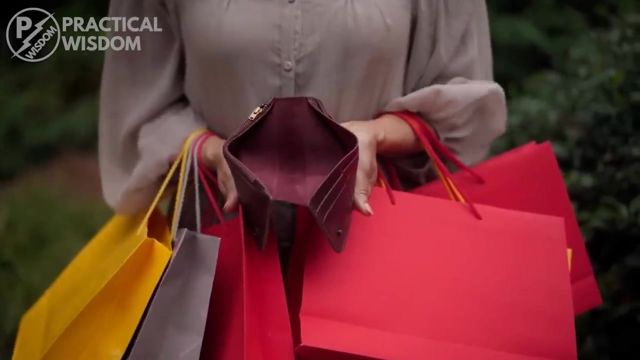 maturity to handle such an instrument. 10. Continue to spend quickly. A spending fast can be just what your personal finances need if you suffer from credit card debt, difficulties, paying payments on time or other financial problems. Basically, going on a spending fast simply means that you're refraining from making any discretionary purchases for a predetermined. 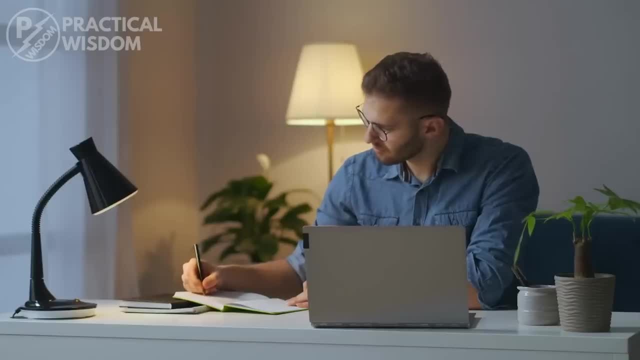 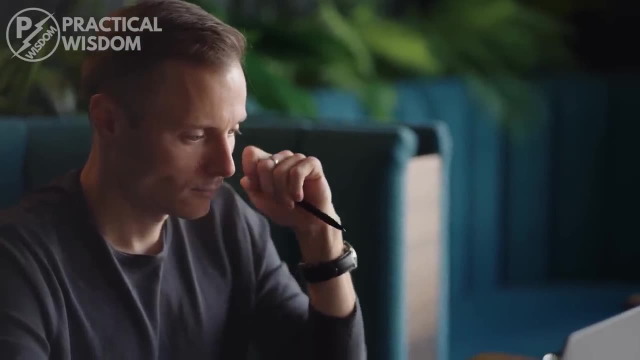 time. This is another great way to help you reduce your spending and get your finances in order. It may sound a bit daunting, but it doesn't necessarily have to be. You may be familiar with the well-known and sometimes contentious detox or cleansing fasts for your body. 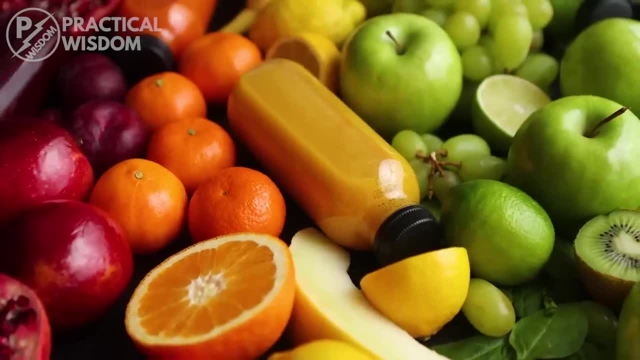 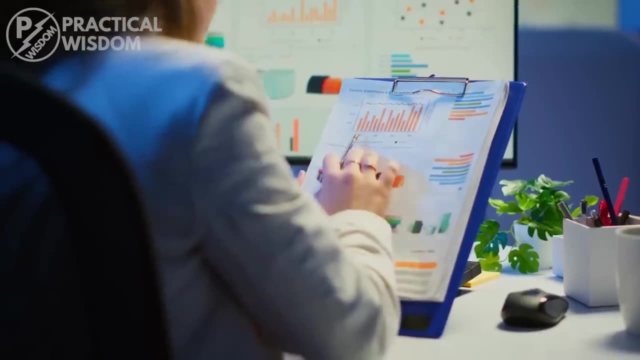 such as giving up sugar or gluten for 30 days or even surviving solely on fruit or vegetable juices for a few weeks. But did you know that in order to achieve financial wellness, you may use comparable fasting or cleansing procedures to your spending and saving behaviors? 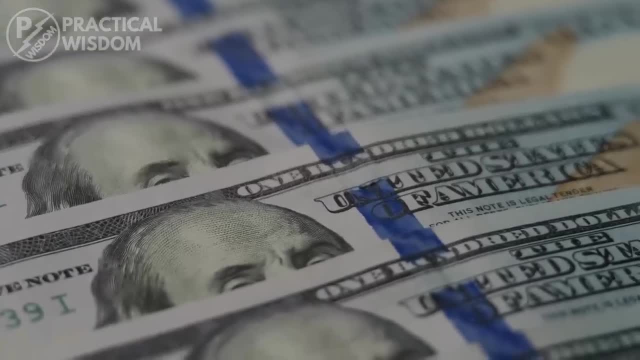 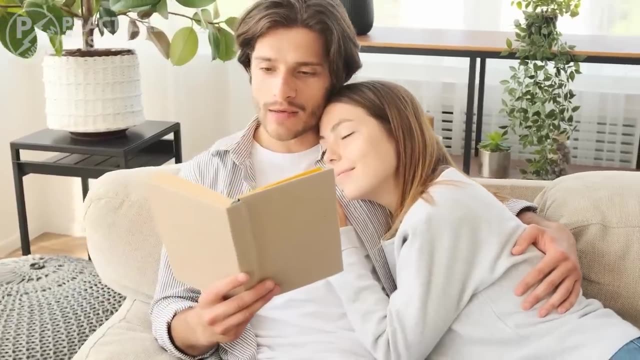 These are frequently month-long periods during which spending and only categories like food, transportation and recurring expenditures are exempted. If you're ready to live simply for a while, commit to this challenge to boost your bank account, alter your behavior and determine what you need rather than just what you desire. 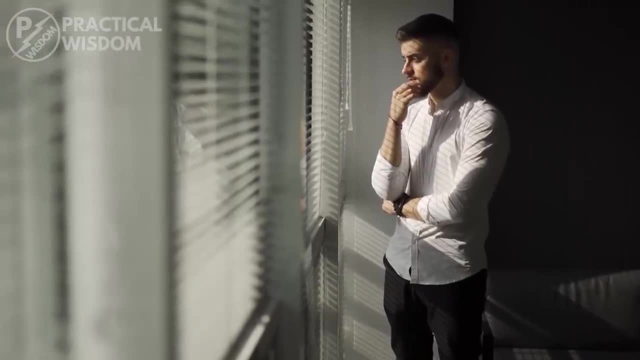 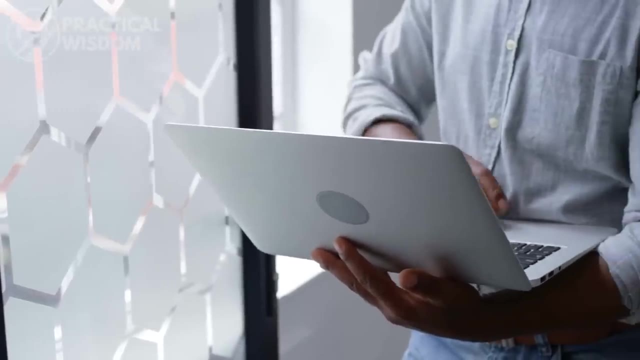 Your perspective on money can even change as a result of the event. It's my hope that this has been helpful to you. Now you can always be one step ahead of your finances by just following the steps from this video. Consider the possibility that you've never had a financial problem. That simply means more money. 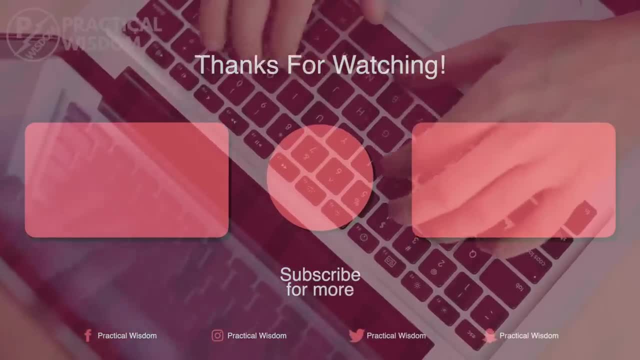 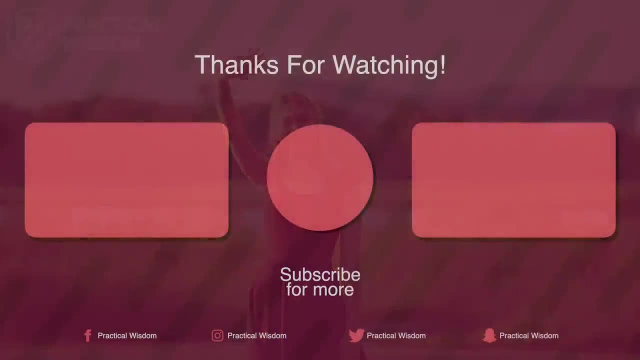 for you. If you have any questions, don't hesitate to leave a comment down below. With that said, thank you all so much for watching. Have a great day and I'll see you all in the next one.